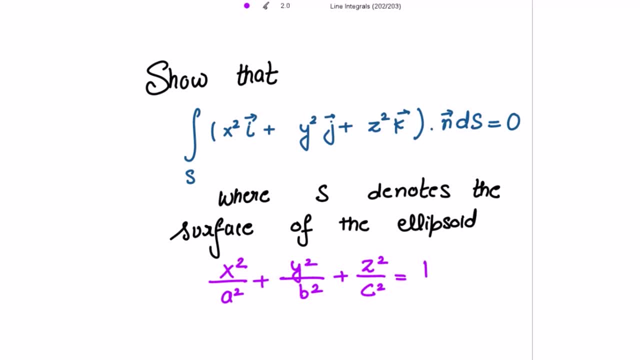 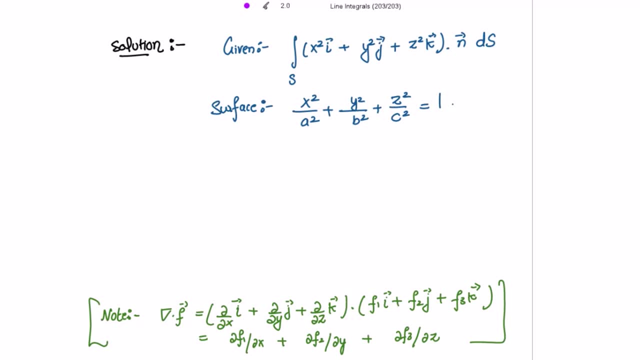 by c square equal to 1.. So we need to apply the Gauss's Divergence Theorem over here. So the given integral is this and the surface is the ellipsoid right. Let's consider the region V enclosed by the surface S, and to solve this surface integral we are going. 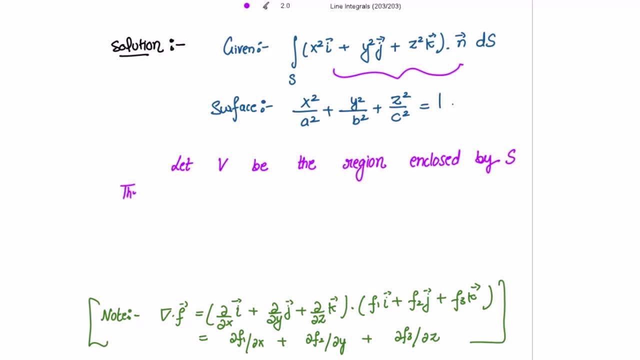 to apply the Gauss's Divergence Theorem. Then by Gauss's Divergence Theorem this surface integral is equal to the volume integral of the divergence of this vector. And for the divergence we write del dot of this vector. Please note over here the divergence. 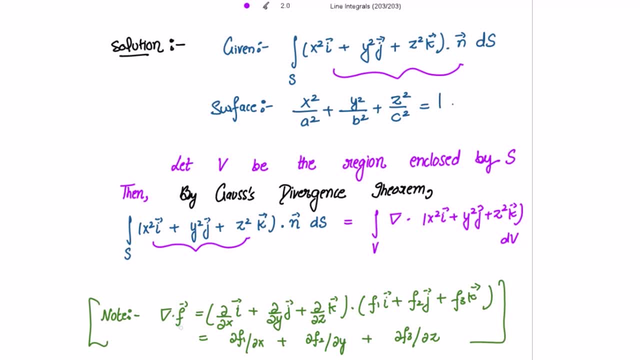 of F vector, that is, del dot. F vector is equal to what is del. It is curly by curly x i vector, plus curly by curly y j vector, plus curly by curly z k vector, And the components of F are written as F1 i vector plus F2 j vector plus F3 k vector. On taking the dot, 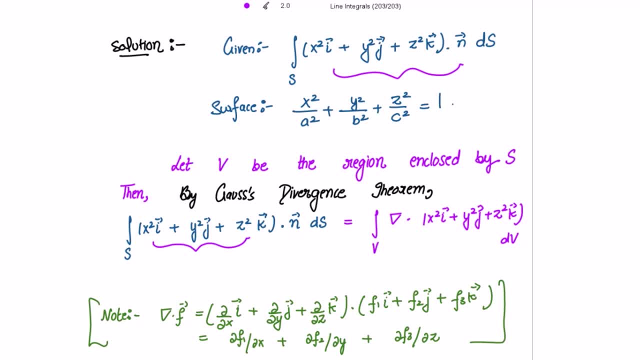 product. we get curly F1 by curly x, that is, that is, derivating the 1 st component with respect to x, plus derivating the 2 nd component with respect to y, plus derivating the 3 rd component with respect to z. This is what 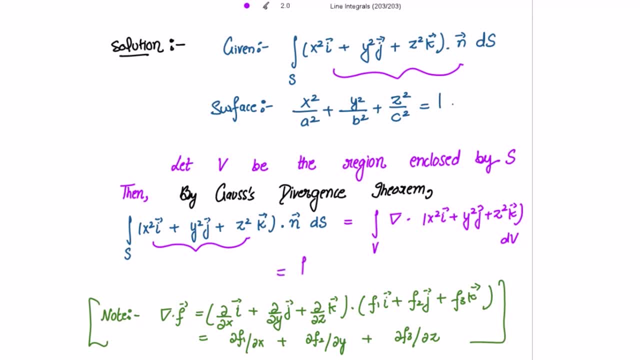 we do over here now. So this is equal to volume integral of-äti fteleri� cat Zi- ≥ f和 fv- fv�jcie理 to z dv. so curly by curly, x of x square is 2x, and then plus 2y plus 2z. so this is equal. 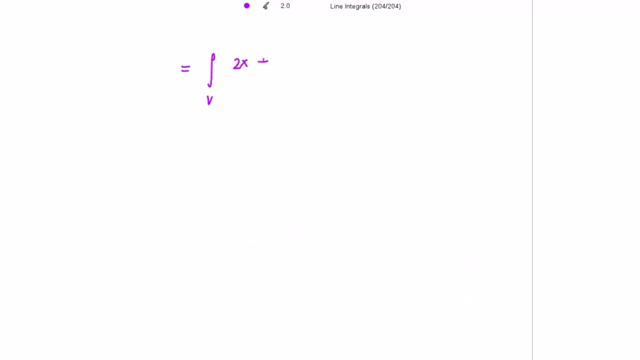 to the volume integral of 2x plus 2y plus 2z dv, taking two common and we get the volume integral of x plus y plus z dv. that is equal to twice of separating the terms, that is, volume integral of x plus volume integral of y plus volume integral of z. now, as we are getting, 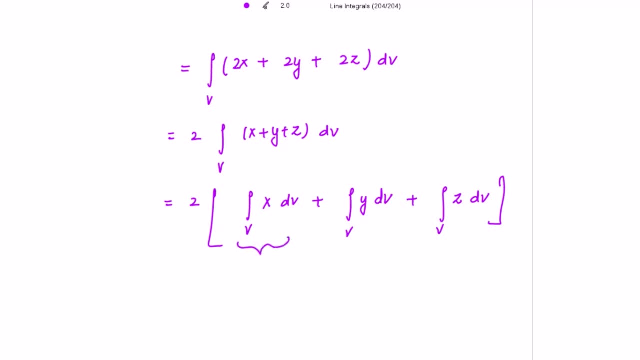 the symmetry. let's solve the first integral, so the volume integral of x plus y plus z, dv, that is equal to the triple integral over the surface s, and the surface s is your ellipsoid: x, dx, dy, dz. now, as the surface given to us is an ellipsoid, that is x square over a square plus. 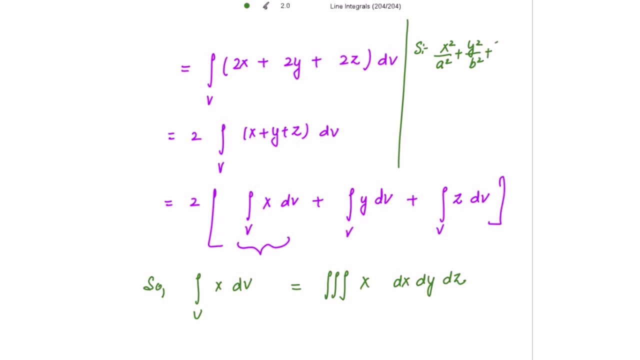 y square over b square, plus z square over c square equal to 1. so we can get the limits of x from here as 1 minus y square over b square, minus z square over c square under the root, with plus, minus sign right. so the lower limit is negative of. 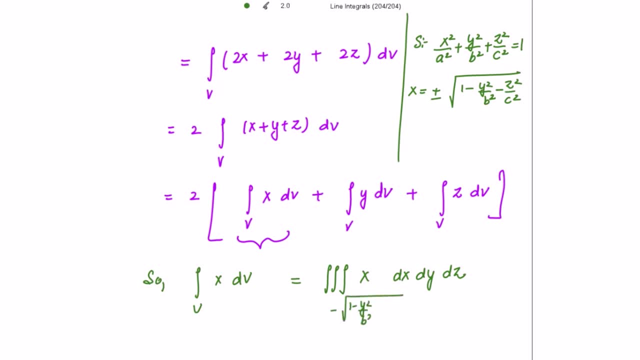 square root of 1 minus y square over b square, minus z square over c square, and the upper limit is positive square root of 1 minus y square over b square, minus z square over c square. right now, this innermost integral is over. we are interesting. 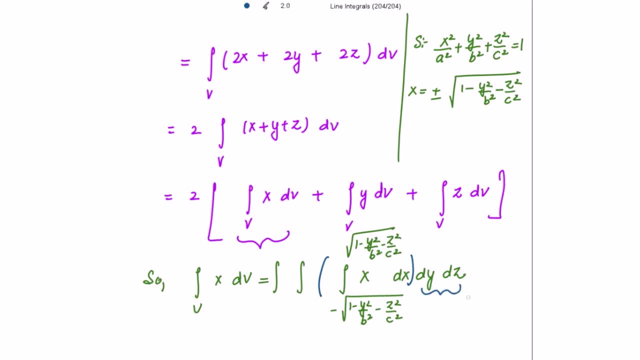 in y z. for y z plane, we take x to be equal to 0 in this surface and getting the limits of y in terms of z. so what we get? so we are getting y to be equal to plus minus 1, minus z, square over c, square under the root. so the limits of y becomes the lower limit is negative. 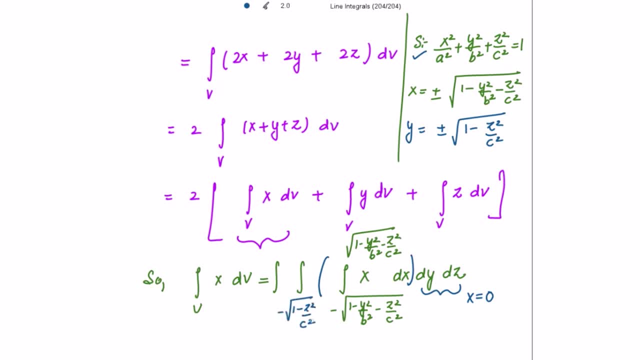 of square root of 1 minus z square over c square, and the upper limit is square root of 1 minus z square over c square. is it fine? ok, alright, now the remaining integral, that is with respect to z. we are interesting in only z coordinates, So for z. 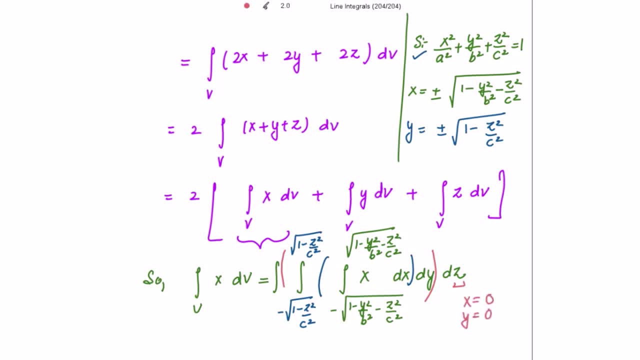 We take x to be equal to 0 and y to be equal to 0 in the surface S and getting the limits of Z. So we get the limits of Z to be, as taking x and y, equal to 0. we get from the surface that it is plus minus C.